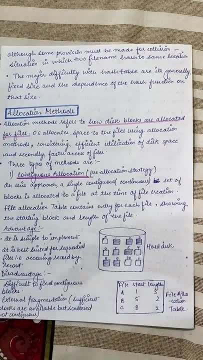 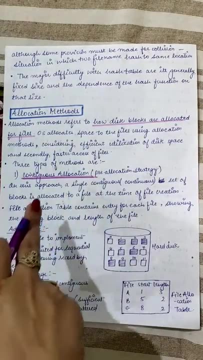 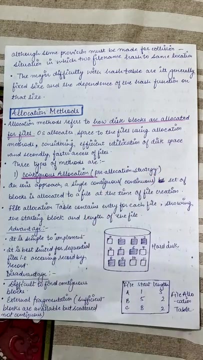 the access of files should be faster. It should be easy to retrieve the files from the data blocks on the hard disk. The three methods we have is: first is contagious allocation. So contagious allocation is also referred to as pre-allocation structure. So the first one is the pre-allocation strategy. So when we were discussing about the memory, 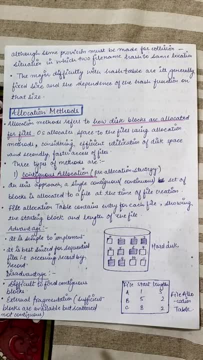 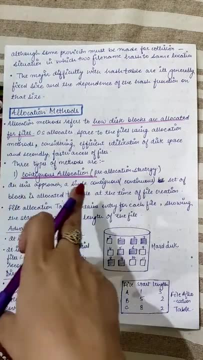 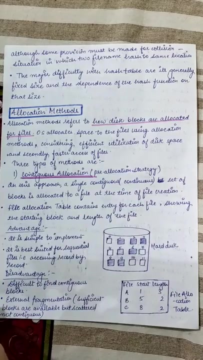 management techniques. we studied about the contagious allocation. We require a contagious, single block Right. So in this approach, also for a file, you will need a single contagious or a continuous set of blocks allocated to a file at the time of file creation. The file allocation. 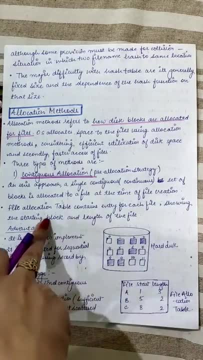 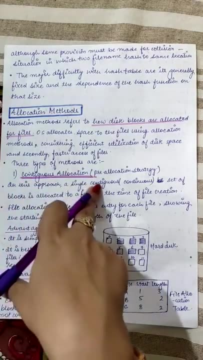 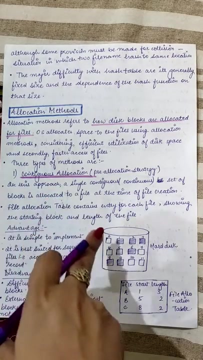 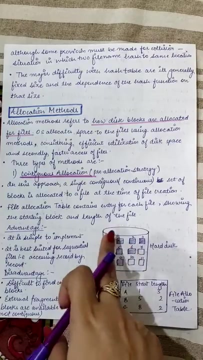 table will contain entry for each file showing the starting block and the length of the file. So contagious block allocation Means that you need to have continuous set of blocks for any file to be stored. Thus you cannot restore the file on scattered locations. So if suppose this is the hard disk and these are the data blocks, okay, where the files will be taking. 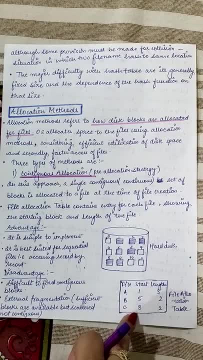 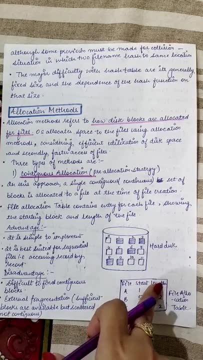 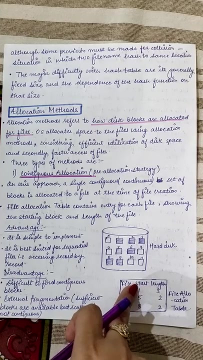 this space And this is your file allocation table fact which has three entries: File, the starting block and the length of the file. that means how many blocks it will require. so if suppose there is a file a, so the starting block of this file is 1. 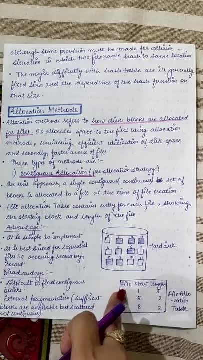 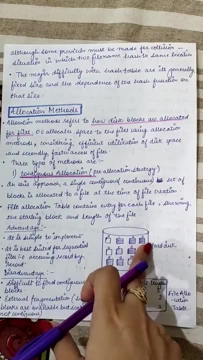 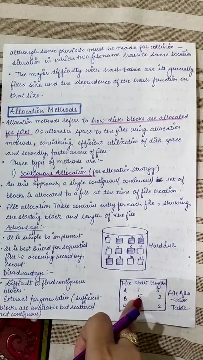 and the length of the file is 3. that means it requires 3 contagious blocks: 1, 2, 3. so all these three blocks are occupied by file a. then there is a file B. a starting block of file B is 5 and it requires 2 blocks. the length is 2, so 5. 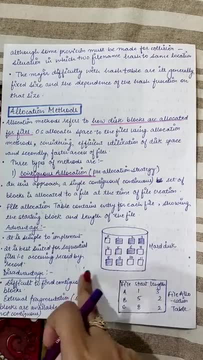 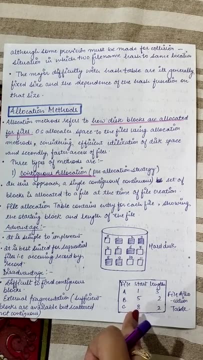 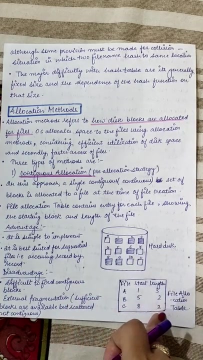 and 6. this is for file B. there is a file C entry in the file allocation table. it starts at 8. that means the block which is start is the block number is 8 and it needs 2 as the length of the file C is 2 blocks. so it will be taking 2 disk blocks. 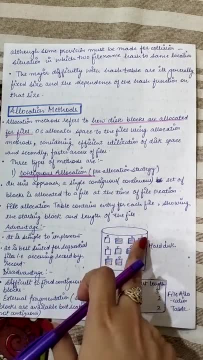 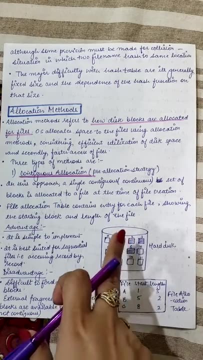 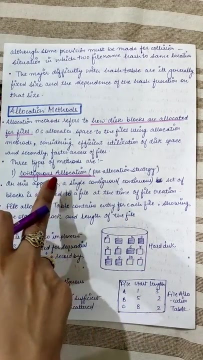 8 and 9 and these blocks need to be continuous. if a file requires 3 blocks, it needs to be continuous. it is not possible that you can have one block on this location, another block on this location, because it is contagious allocation. got the idea. now we have advantages and disadvantages of contagious allocation. the advantage: 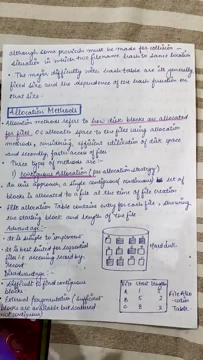 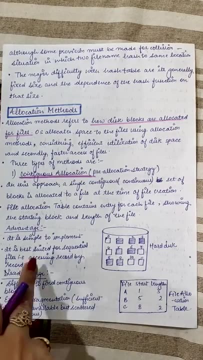 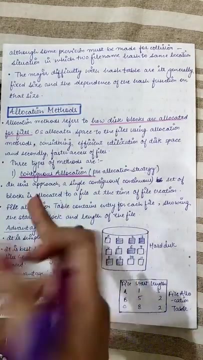 is that it is simple to implement. all right, it is simple to implement. you just need to provide the continuous allocation space sequentially. and it is best suited for sequential files because in sequential file access you have record by record, one after the other access, so here you have continuous. 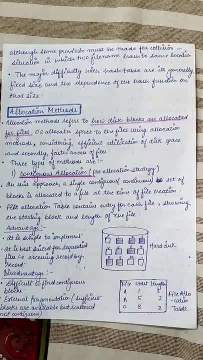 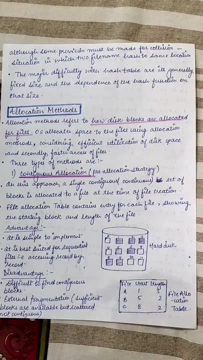 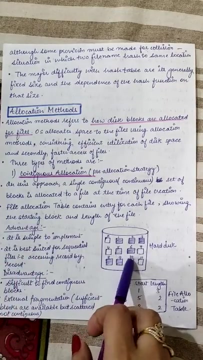 blocks so you can easily access the files in a sequential manner. the disadvantage is that it is not always possible to find the contagious blocks. if you have another file, file D, which requires three blocks, then you can easily give the three blocks, but there are no three blocks available. 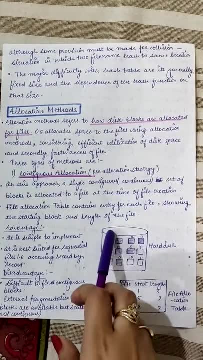 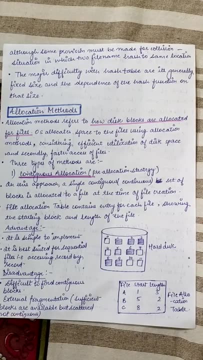 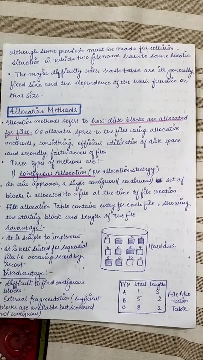 continuously. there are two blocks here, one block here, one block here, but it is a contagious allocation, so you need three blocks together, which is not possible, right? so it is not always easy to get the contagious blocks. and secondly, this approach is suffering from external fragmentation. I have just shown 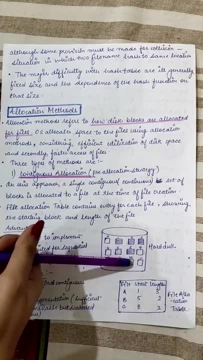 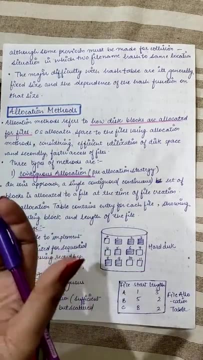 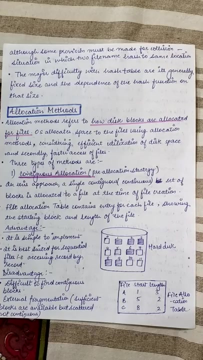 that you are having these disk blocks available to be allocated, but the operating system cannot allow this to happen. you cannot allocate these blocks to the file requiring three blocks in a continuous fashion. all right, so this is external fragmentation. next, we will be discussing about the linked allocation. the linked allocation is a non contagious 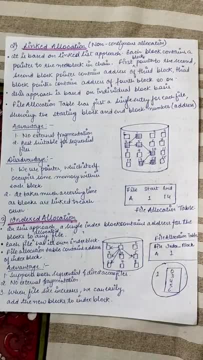 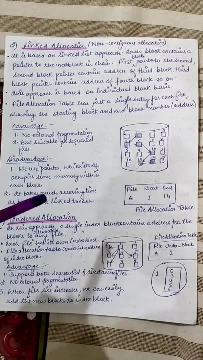 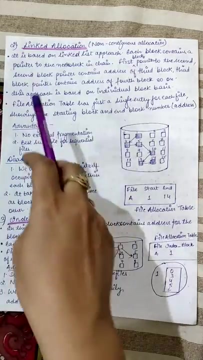 allocation. that means you are not looking for a continuous block sets available, all right. it is using a list and it has a linked list type of approach. that means if the blocks will be pointing to the next block, all right. so it is based on linked list approach. each block contains a pointer. 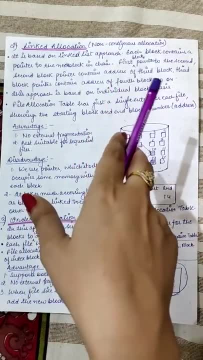 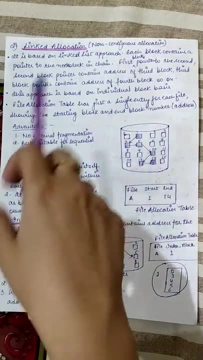 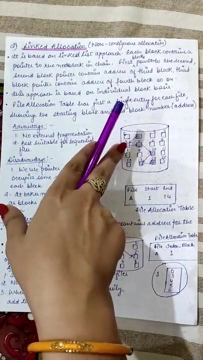 to the next block in the chain. first block points to the second block and second block points to the address of the third block. third block contains the address of the fourth block, and so on. this approach is based on individual block basis, because every block is containing the address of the next block. 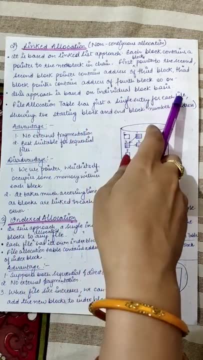 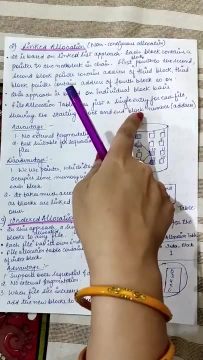 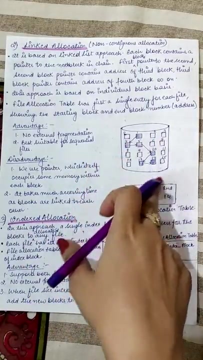 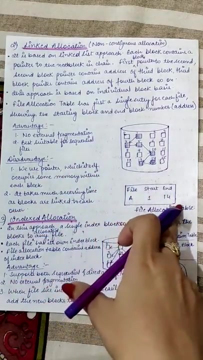 the file allocation table has a single entry for each file showing that the showing the starting block, where the file block starts, and the end block number, right? so if this is the diagram of your hard disk according to linked allocation, then there are again. you have 16 blocks available, addressed from 0 to 15, and there is a file allocation table which 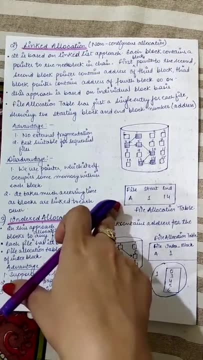 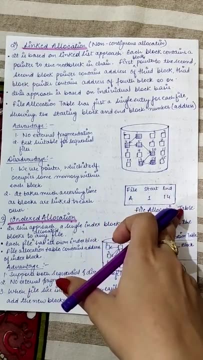 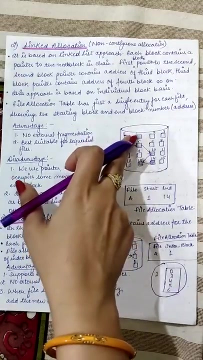 has three entries: file a- this is the name of the file- the starting block once it's started, and then the end block where the file ends. so this file starts with a starts with 1. sorry, so a file starts with 1 as the first address of the block. so 1 contains the address of the next. 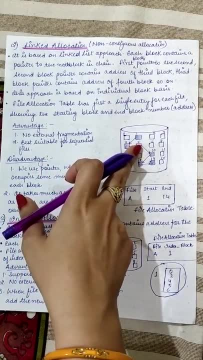 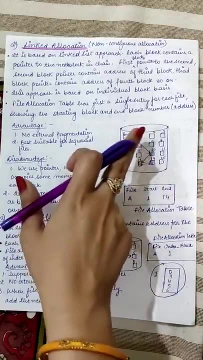 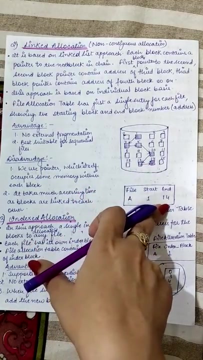 block, which is 4, 4 points to 5. next address is of 10, 10 points to 13, 13 points to 14. that's why the starting block of the file a is 1, address is 1 and the end is 14. so this is the linked allocation. every data block is. 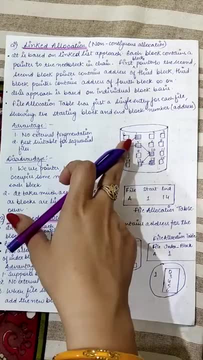 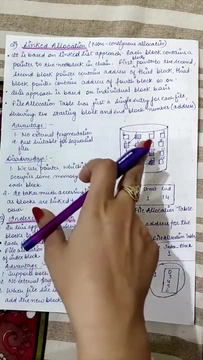 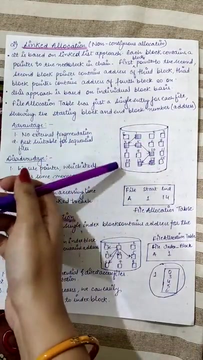 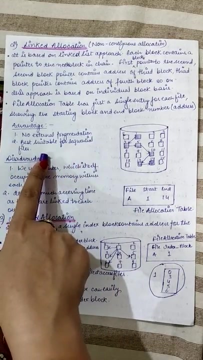 linked to another block. that means through pointer it contains the address of the next block. advantages no external fragmentation because here one block is containing the address of the next block, so you can use the non contagious approach over here, so external fragmentation will not occur. it is best suitable for sequential files in which the records are accessed one after the. 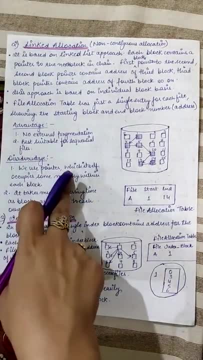 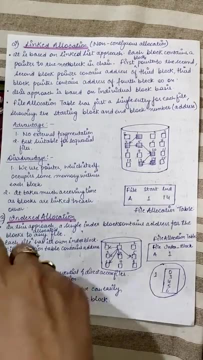 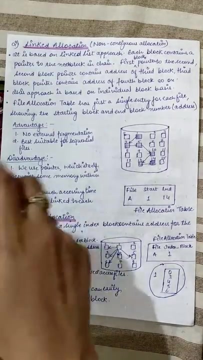 other. the disadvantage over here is that we are using pointers, so the pointers will also require some memory within each block. so that will take space and secondly, it takes much accessing time. as blocks are linked to each other, the access time is more because every block is linked to every other block. thus if you have hundred blocks, then you will be 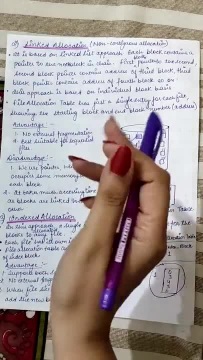 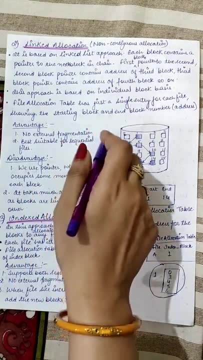 accessing every block. so that is the disadvantage over here. so in this whole process we defined the block as the indexed block and the indexed block is the indexed block in the indexed block is the indexed block. now, if you want to access 99 block, there is no way that you can raise. 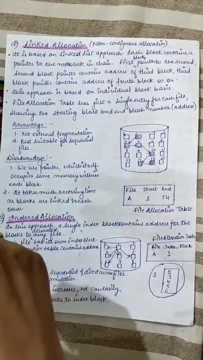 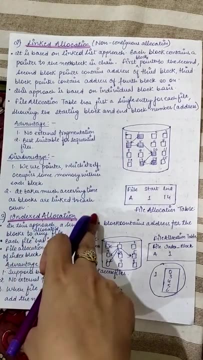 the 99th block directly. you will start from the beginning of the file and then from one pointer to next pointer, then next pointer, then you will raise the 99th block. so the disadvantage is that only that we are using the pointers over here, which needs the memory space. 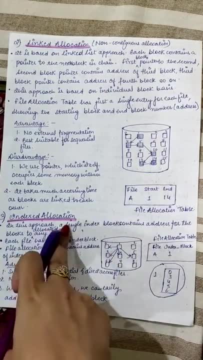 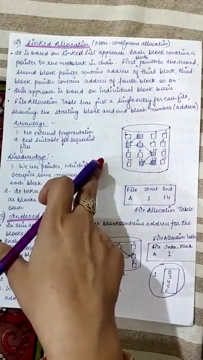 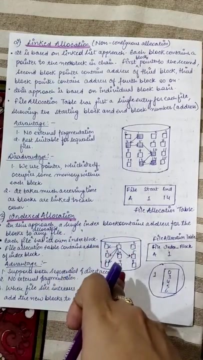 again in the block- secondly, the access time is high- contains the address for the blocks to allocate to any allocated file. so in this we had every block containing the address of the next block. but in case of indexed allocation what we do is suppose this is the hard disk diagram and there are total of nine blocks, zero to eight. so this: 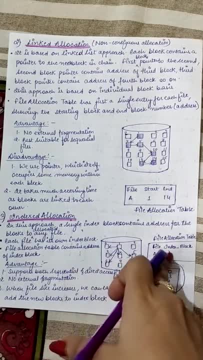 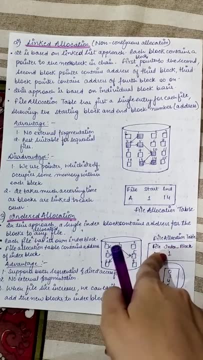 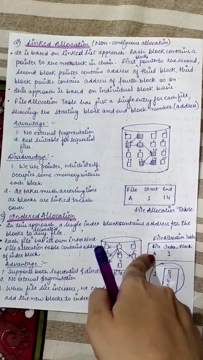 one is labeled as the index block. okay, in the file allocation table there are two entries. only one is for the file name, file a, and there is an index block. it is one. so this one block contains the pointer to all the blocks used by file a. all right, so here we are not connecting one block to. 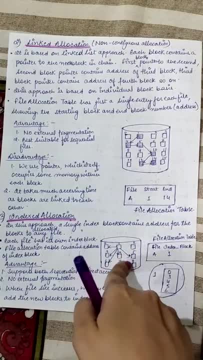 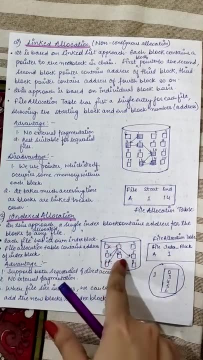 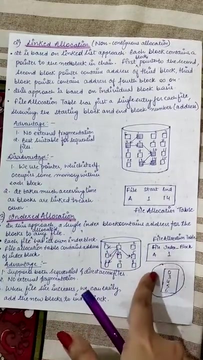 the next block, next block to the third block address, third to the fourth block address. but what we have done is that we have taken the first block as the index, which contain all the other blocks entry. so this is your file. a index block is one and this index block is being shown over here. that one is connected to zero one. 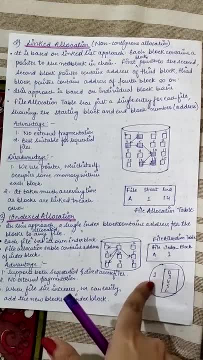 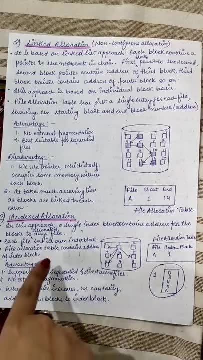 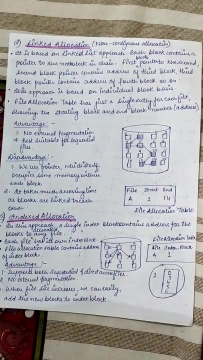 is also having a link to three, one to four, one to five, one to six. so each file has its own index block. every file will have its own index block. file allocation table containing the address of the index block. advantages is that it supports sequential as well as direct access. so sequential. 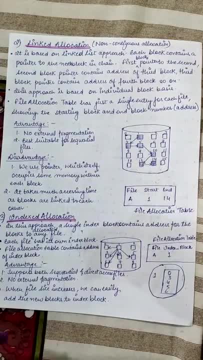 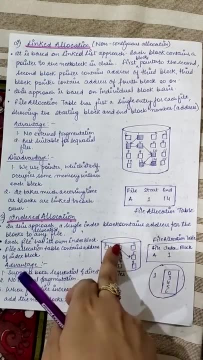 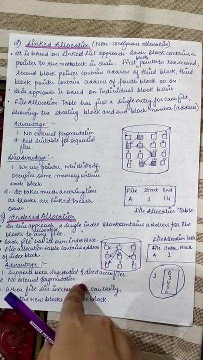 access is also possible, which was also possible in our earlier two cases, but it supports direct access. if you want to go for the block number six, then from one there is a direct link to six, so you can access that block directly. there is no external fragmentation because we do not need. 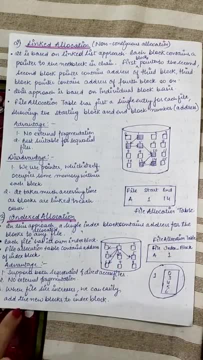 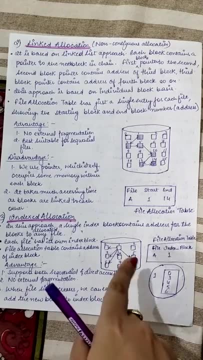 the continuous set of blocks. when file size increases, we can easily add the new blocks to the index block. and this is also possible- that if you want to add the new blocks, suppose you add some information to the file, you add the content to the file, then the new block will be.